Not all businesses require a ton of capital to get started. In fact, some can be started for an investment of $5,000 or less. If you have a mind to start an eco-friendly business, here are some $5,000 sustainable business ideas you can implement in order to save the planet. 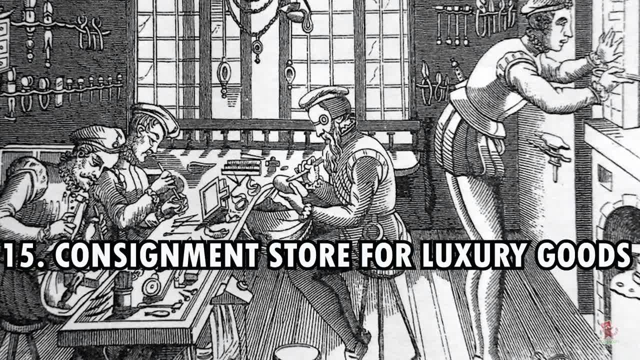 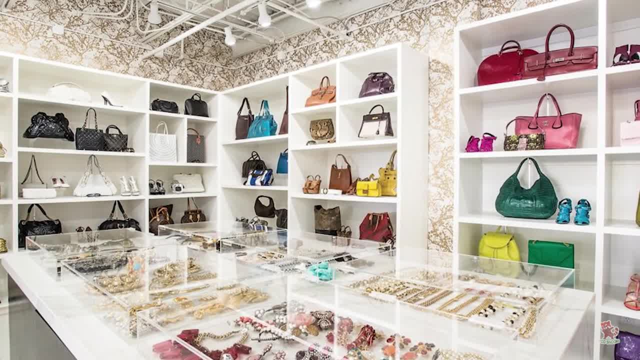 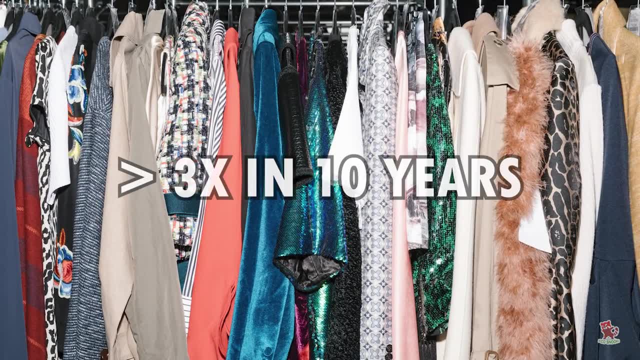 Merchants have sold upscale secondhand clothes and accessories since the Renaissance era, and today it's a flourishing, sustainable business idea. In fact, the secondhand clothing market in the US is projected to more than triple in value in the next 10 years. As a consignment retailer, 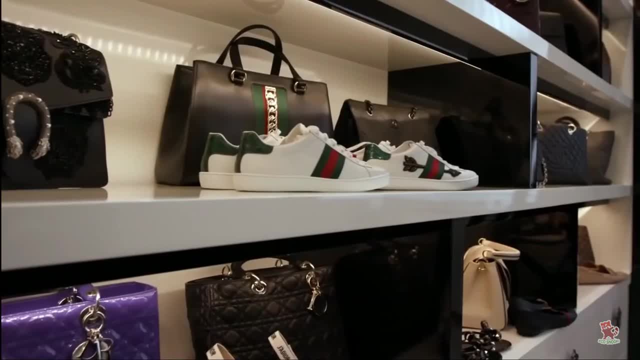 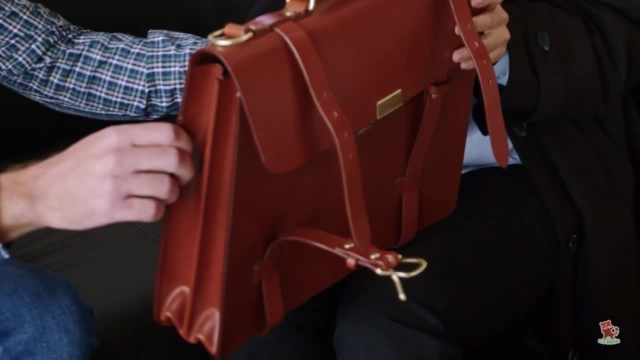 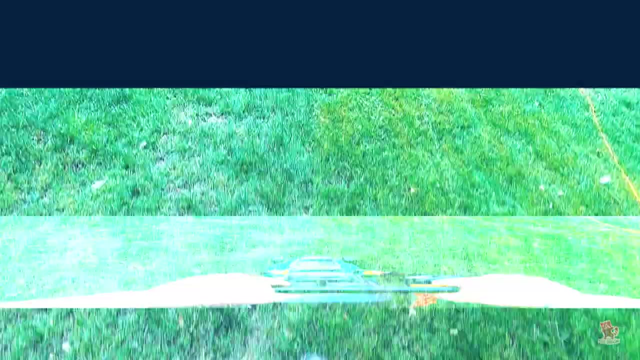 you agree to give a percentage of an item's sale to the first owner of that particular item after you sell it for them, And the eco-friendly upside is that, unlike traditional retail stores, you don't need to purchase inventory. Lawn Care Services is one of the home. 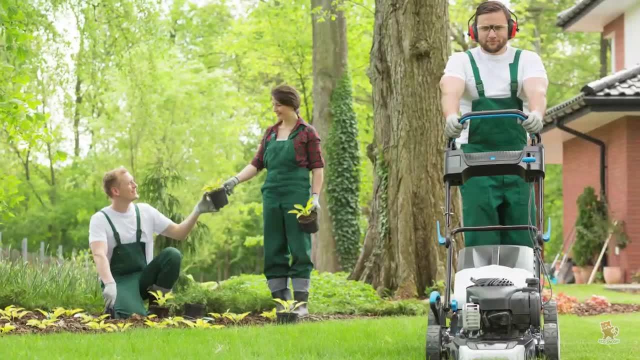 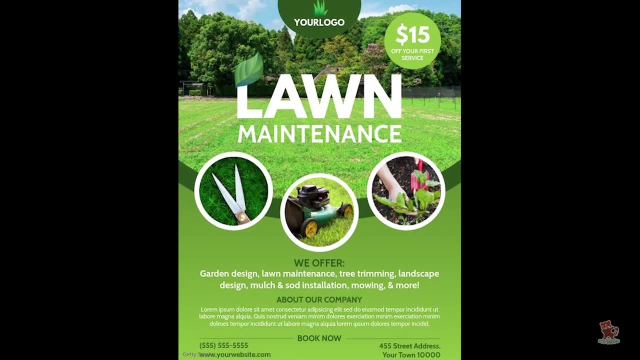 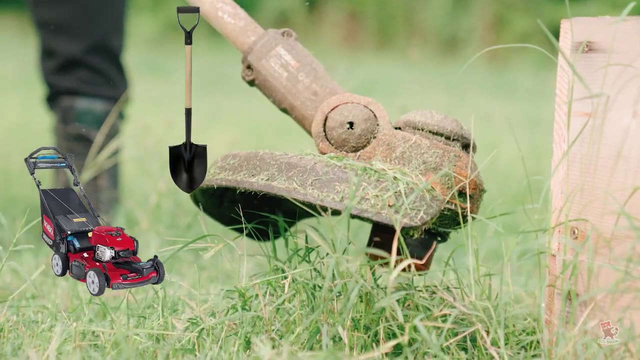 improvement cum green, service-based business that an entrepreneur who is interested in making money should consider starting. It is a business that is easy to start and manage. The basic equipment needed to start this business are lawn mower, shovel, rake, wheelbarrow, shearer and sufficient. 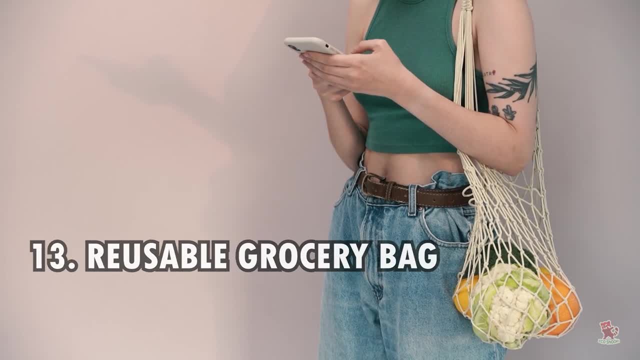 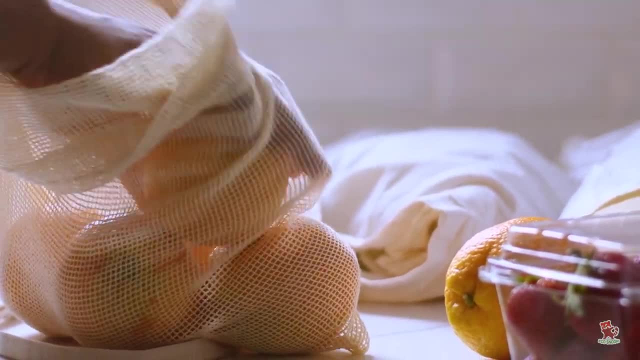 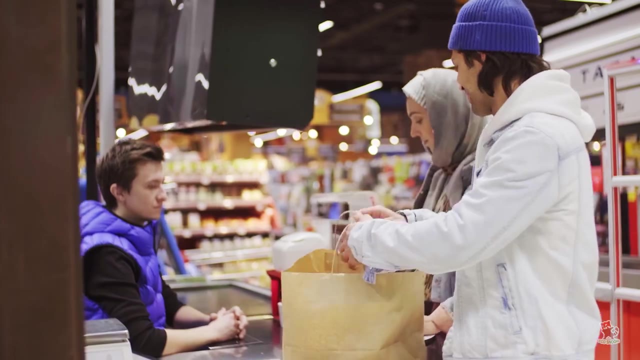 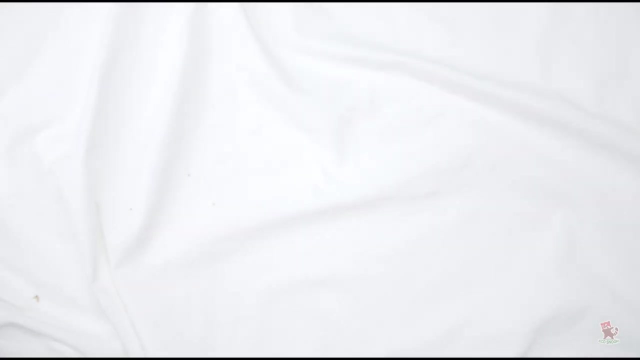 labors. A reusable grocery bag business looks to supply durable and decorative grocery bags designed for multiple uses to help reduce the reliance on plastic grocery bags. As more consumers decide to ditch the plastic bags, options for reusable shopping bags will become more and more popular. Some stores already require customers to bring their own bags with them for 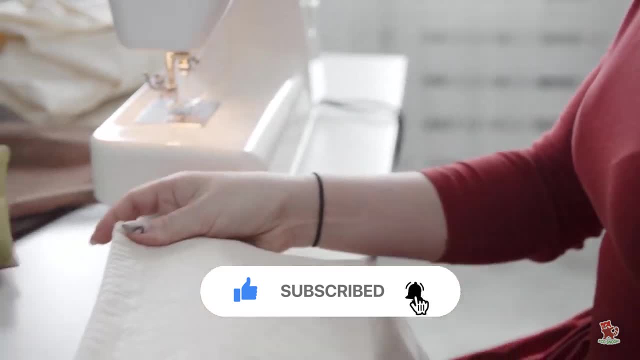 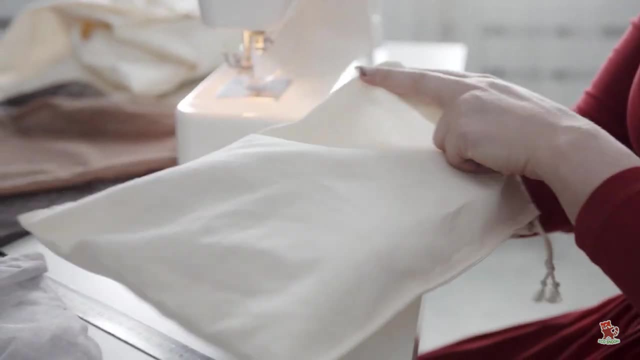 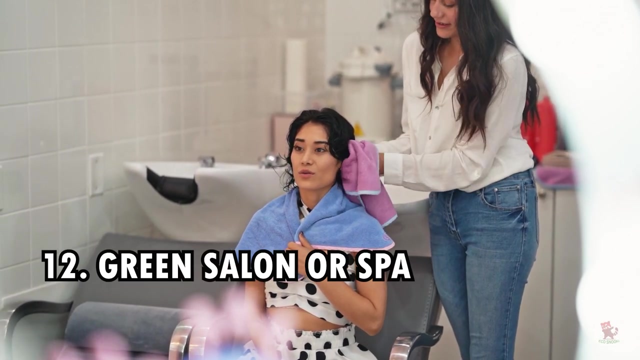 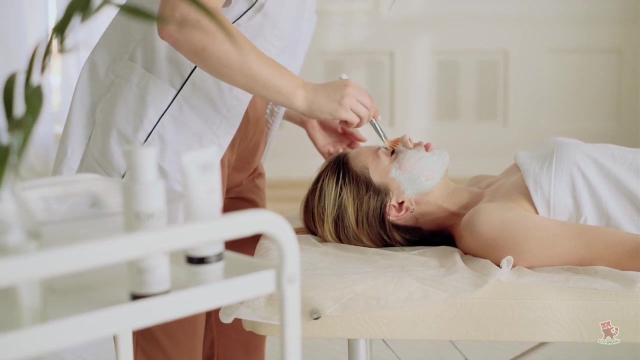 their shopping experiences. Reusable grocery bags are a great example of eco-friendly products that helps make consumers' lives easier and less wasteful. Entrepreneurs interested in the beauty industry could open a salon or spa that specializes in green practices, including using products without toxic chemicals, give herbal remedy and apply Ayurveda. 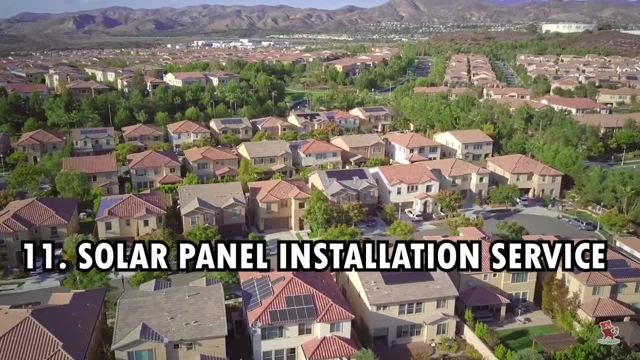 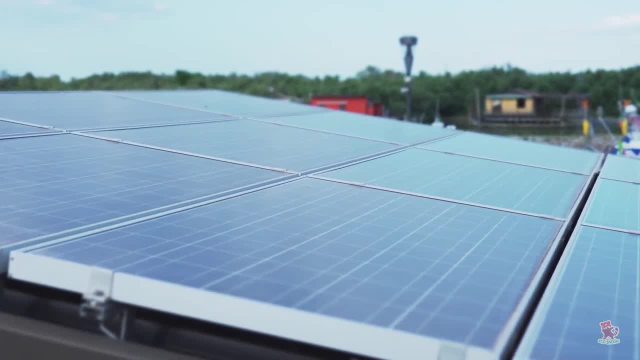 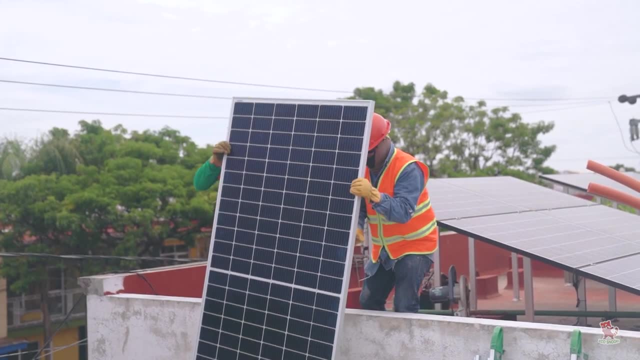 Many green-minded homeowners have installed solar panels on their homes and many more would like. If you know how to do this, offer this service in your area. It is also cheap to buy solar panels. An entrepreneur can exploit this and deal in solar panels. 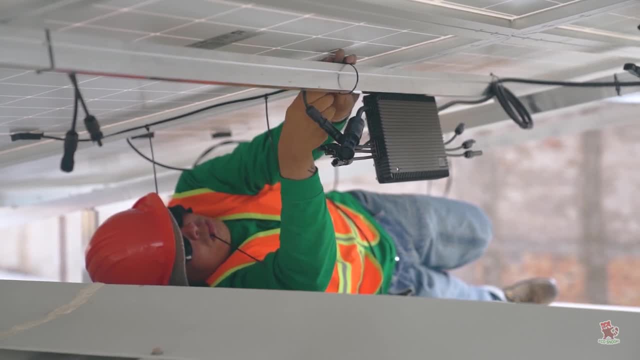 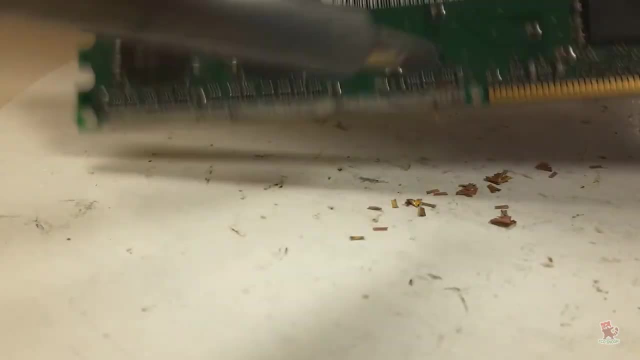 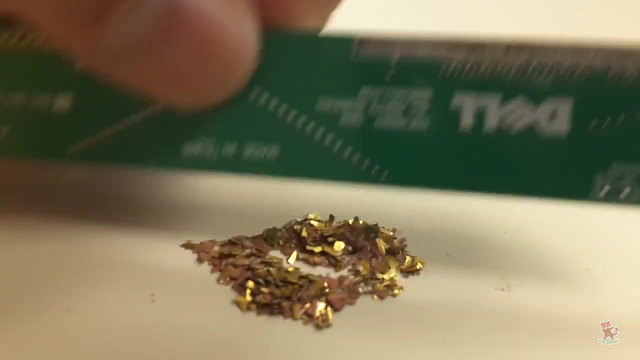 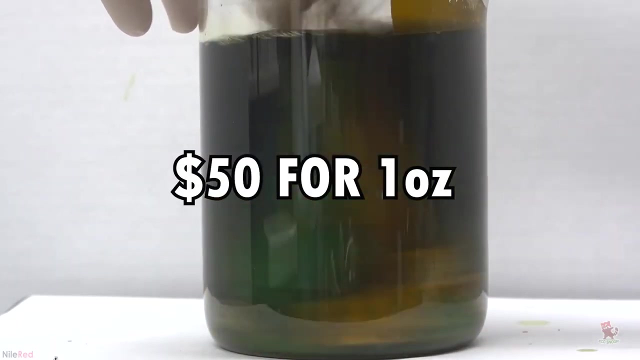 and also offer installation services at a fee. The recovering and selling of scrap gold is yet another profitable and thriving small scale green business idea that an entrepreneur can successfully launch. You can start right from where you are. The good thing about this process is that it would only cost you about $50 to recover one ounce worth. 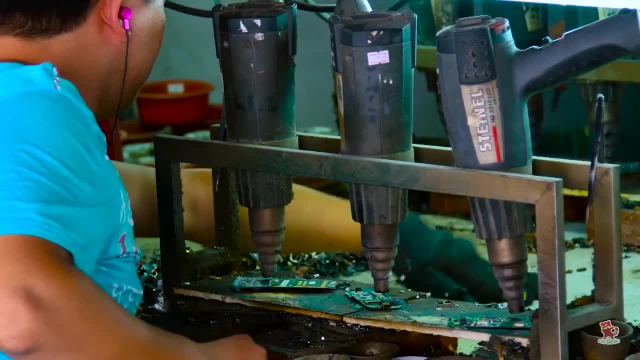 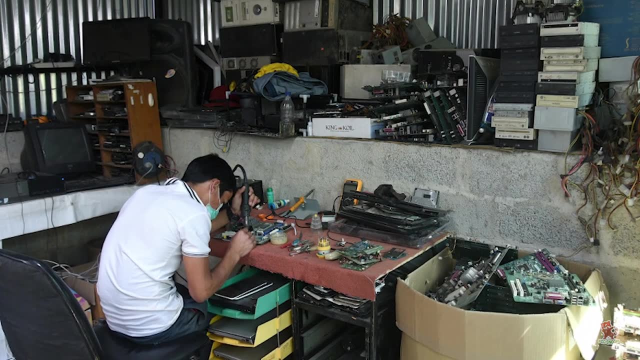 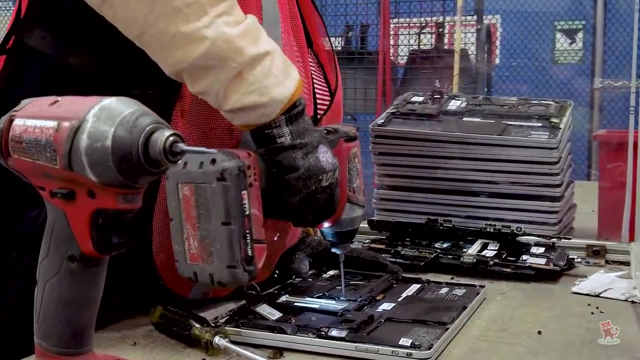 of raw materials. The good thing about this money-making venture is that you can get the raw materials for free, Because the electronics repair shops would see you as a helping hand for its disposal. The basic requirements needed to start this business are some tools to recover. 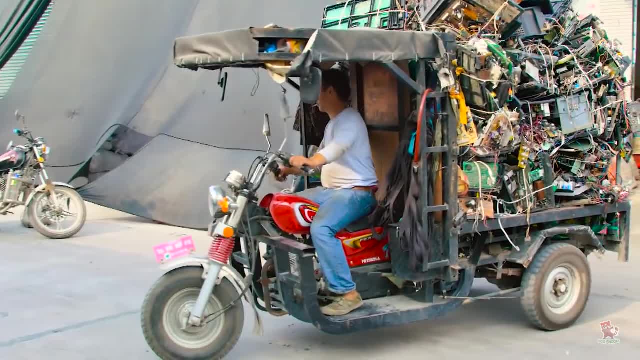 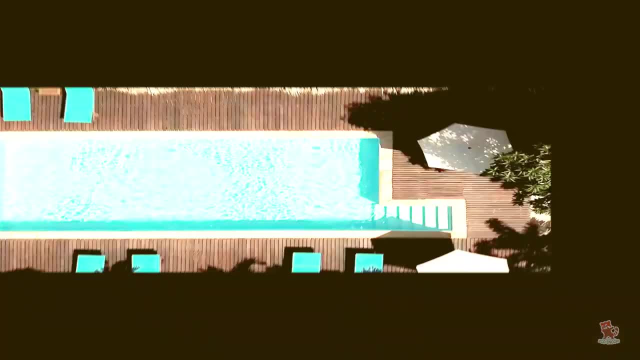 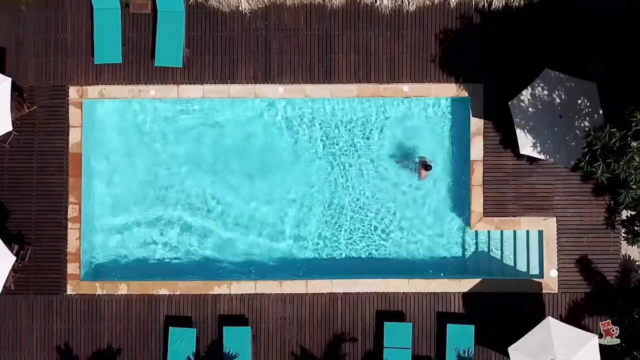 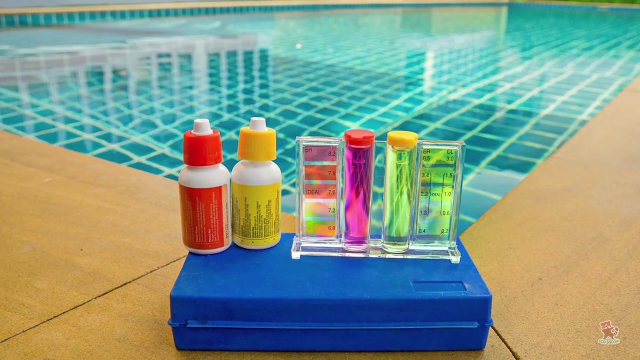 gold from PCBs, a small goods vehicle to collect the raw materials, sufficient manpower and a work area. The swimming pool industry is expected to grow by more than 25% in 2025. So this niche is in high demand. Since chlorine is considered a pesticide by the EPA, you can 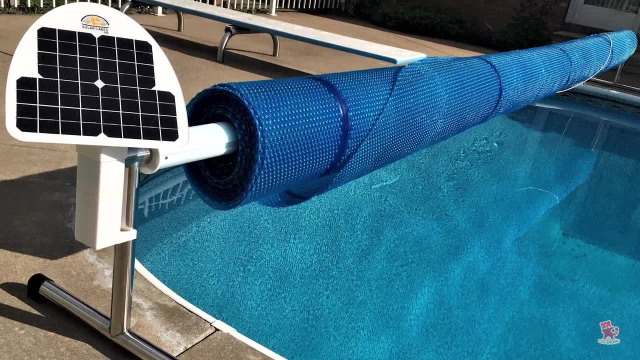 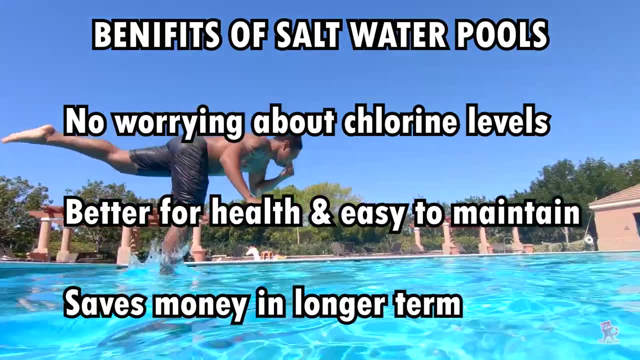 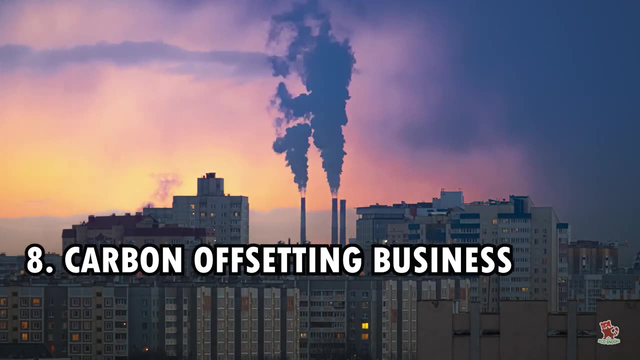 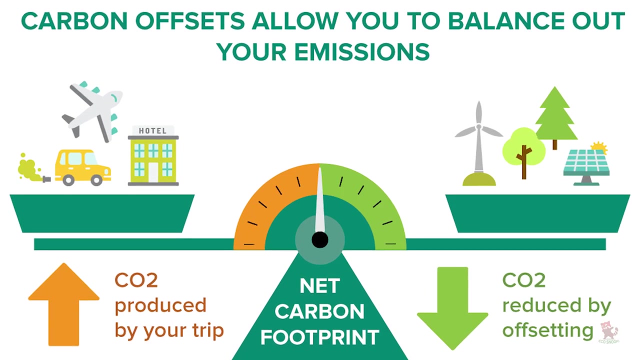 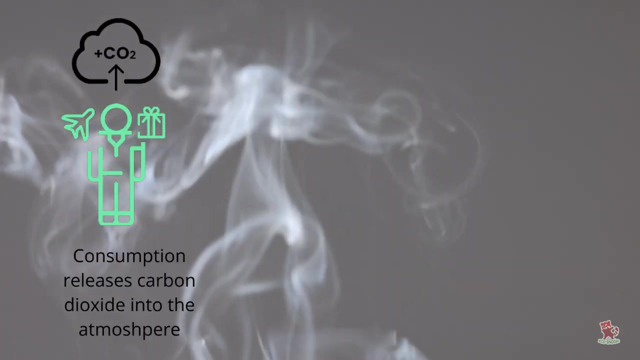 offer your clients green cleaners, install solar pool covers and help them switch to saltwater systems. Carbon offsetting is the practice of purchasing carbon credits for carbon dioxide emissions, which in turn, help fund projects to reduce carbon dioxide in our atmosphere. This practice works to reduce the carbon emissions and carbon footprints of businesses. 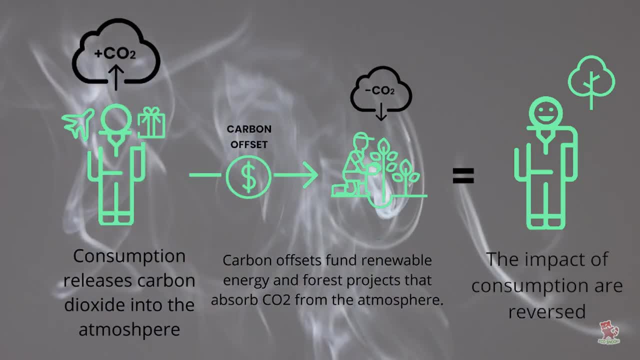 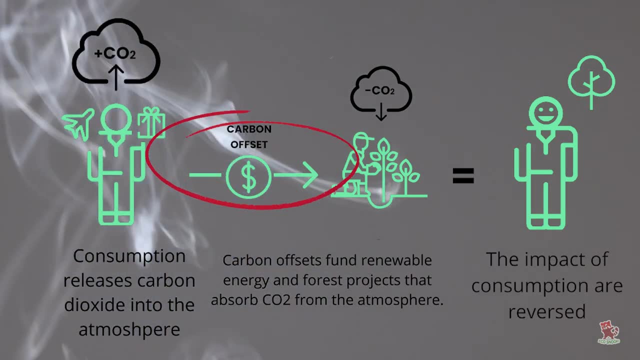 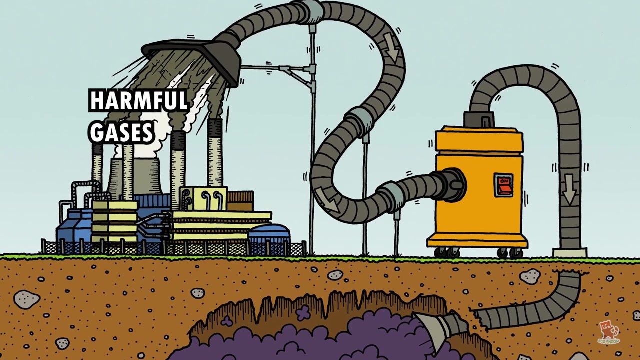 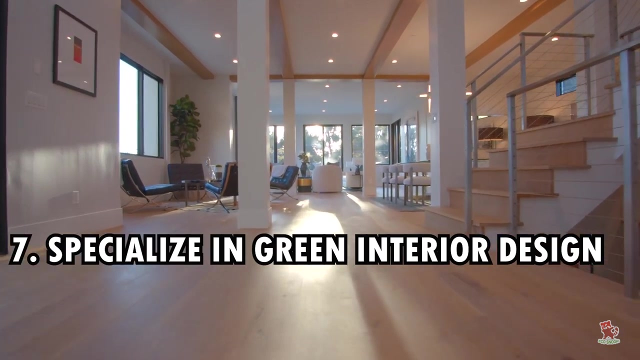 and organizations. In essence, a business buys out their carbon emissions by paying a fee which goes to fund programs and initiatives that work to support renewable energy plans and methods, or waysisk d, to capture harmful greenhouse gases such as methane. Interior designers can use sustainable fabrics, appliances and furniture to improve indoor air. 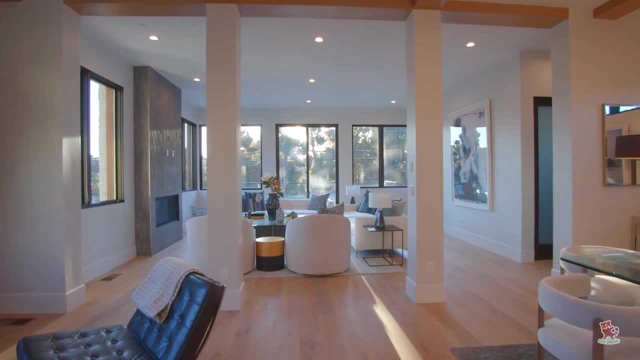 quality and reduce clients' electricity bills while keeping the environment safe. For example, America loses 31,000 square miles, or 30,000 square miles a year, for human waste. app Senate of North Africa, who recorded in Suburban Air inglés, new statement. 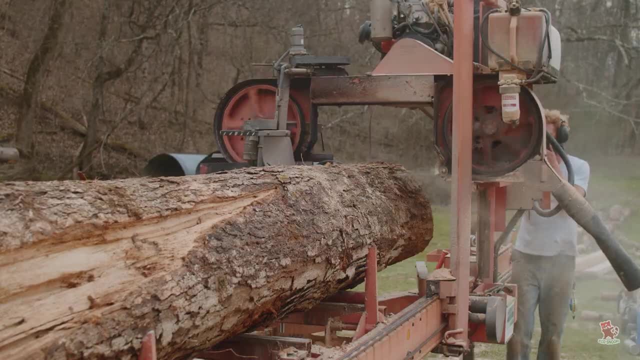 would be喜arse of the climate emergency. longer term, when he joining the administration, will lift more flies' energy returns, leaving sustainable milieu, and also streamline the economic landscape of forest to deforestation annually. You can help people choose sustainable flooring materials such 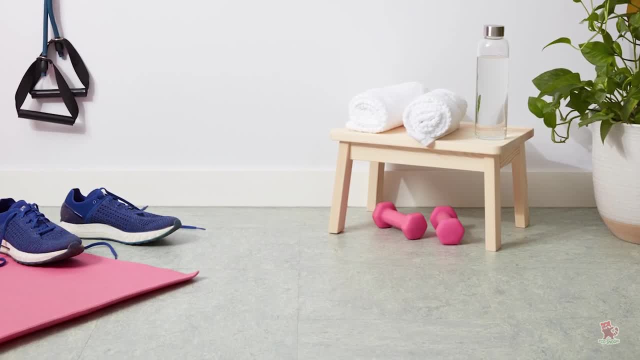 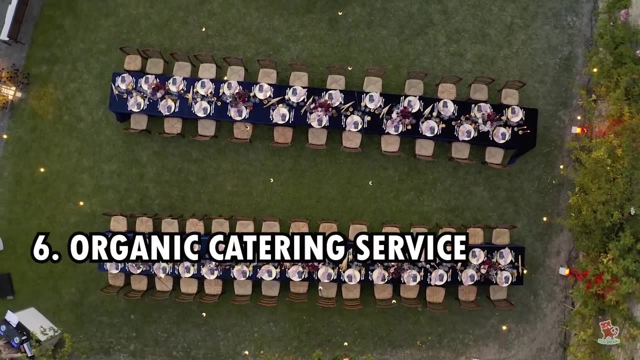 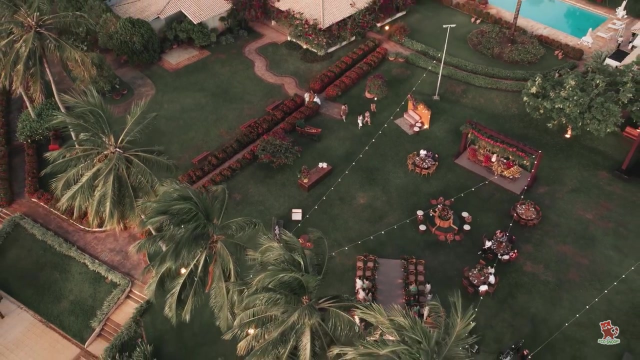 as bamboo, cork and natural linoleum. A great way for eco-friendly foodies to share their passion for food and the environment is to start an organic catering company By catering local events and business luncheons with foods containing organic and locally grown ingredients. 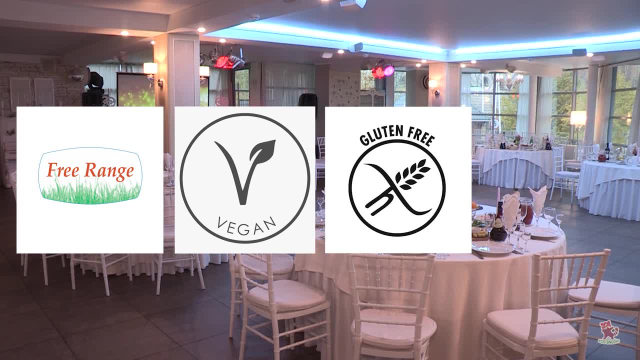 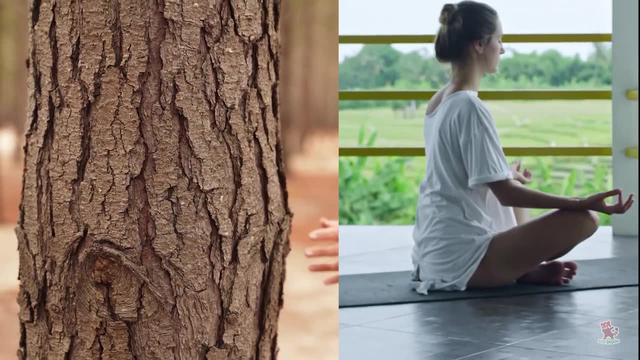 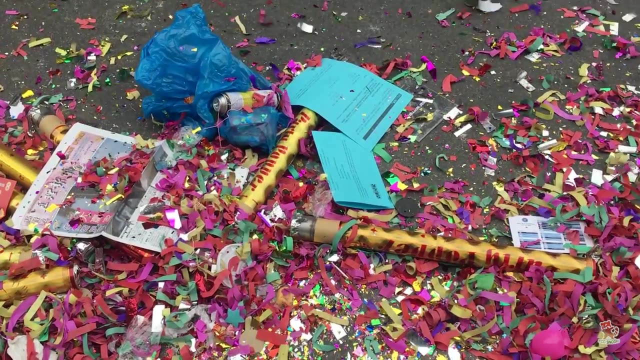 free-range meats and vegan, gluten-free and paleo meal options, you'll appeal to nature lovers and health and wellness enthusiasts alike. Be sure, though, to minimize the impact on the environment by avoiding plastic and paper goods as much as possible and composting food waste. 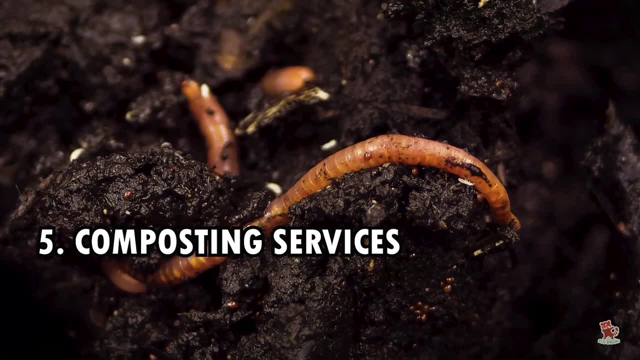 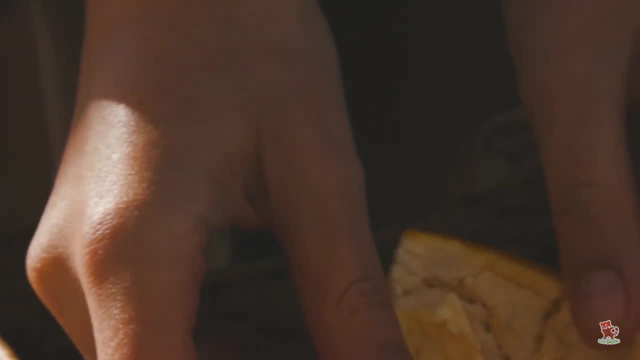 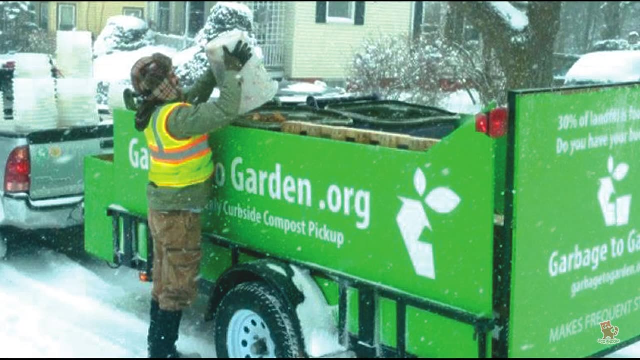 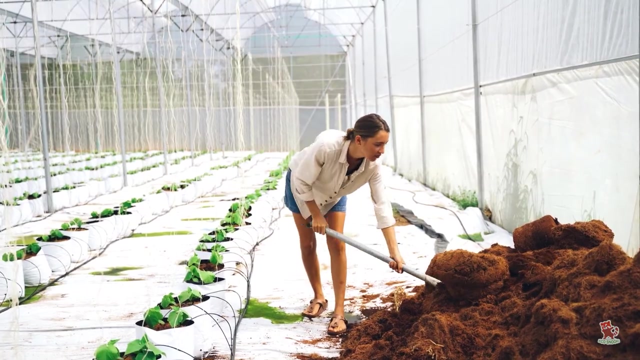 Worm farming and organic compost sales are other green gardening business ideas. Some consumers may be interested in composting food waste to help the environment, but not all of them have a use for the end result. You could start a business that collects composted material from homes or businesses and sells it to gardeners or farmers. This is a move that ensures their 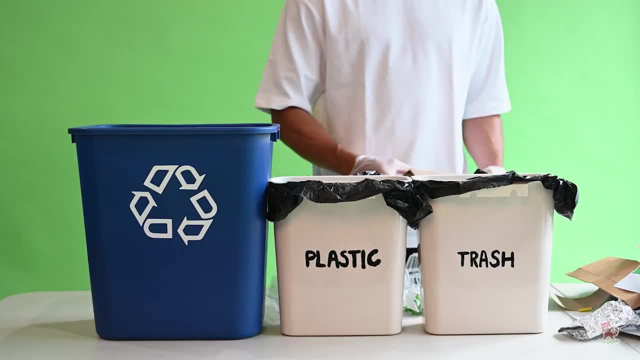 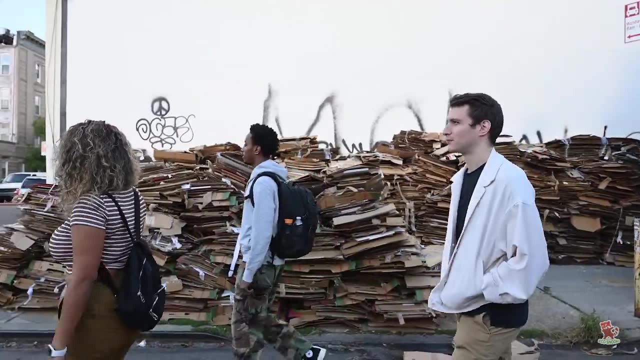 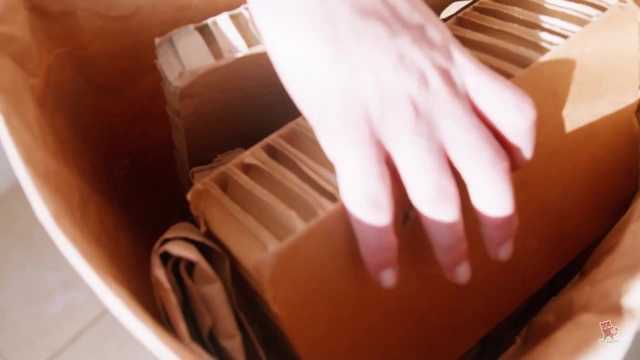 is the optimal use of the cardboard by recycling those that would go to the landfill or already in the landfills. plus, there is a lot of waste cardboards lying around, which pollutes the environment. thus, the business of recycling means less waste in the land and creates an opportunity. 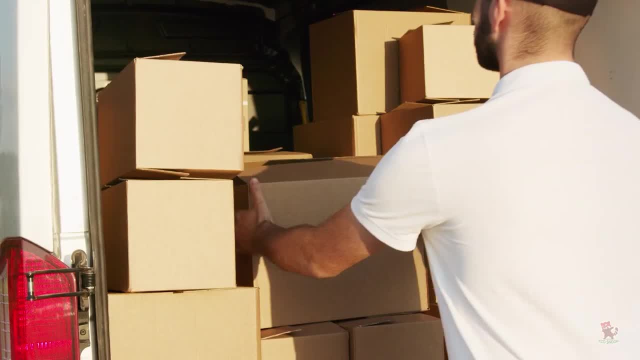 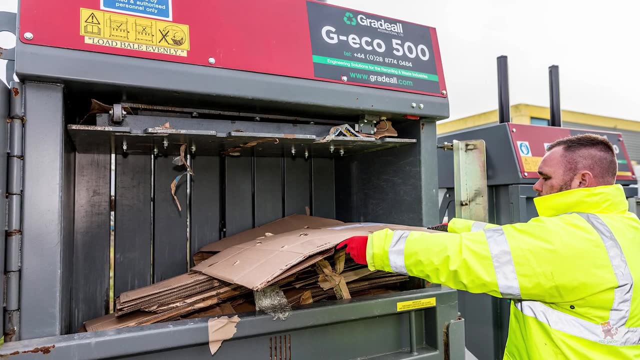 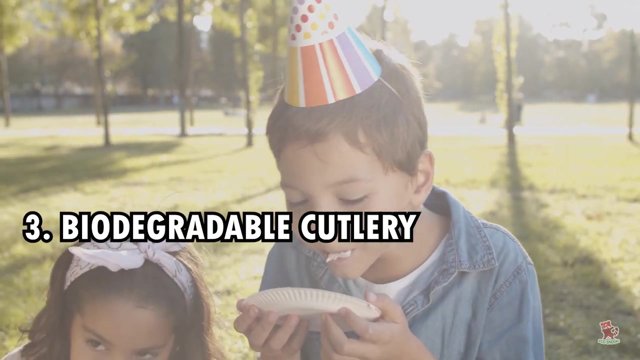 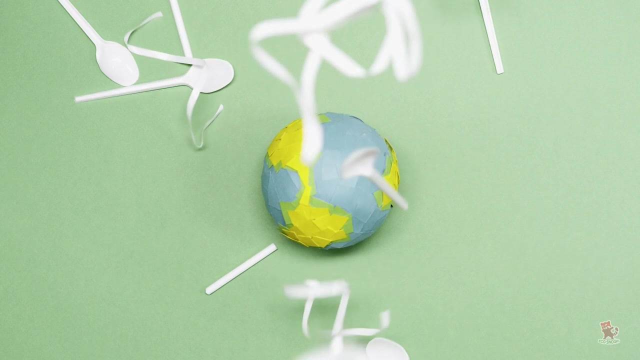 for people to make a living from the process. cardboard can be recycled for reuse and can be used in the manufacture of cardboard related materials such as books. the normal paper plates and plastic cutlery that is available in the market are extremely harmful to the environment. the plastic spoons, forks, and paper plates and cups add to the rising waste on the planet and 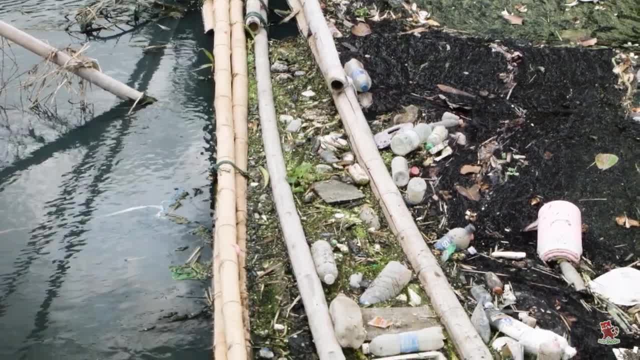 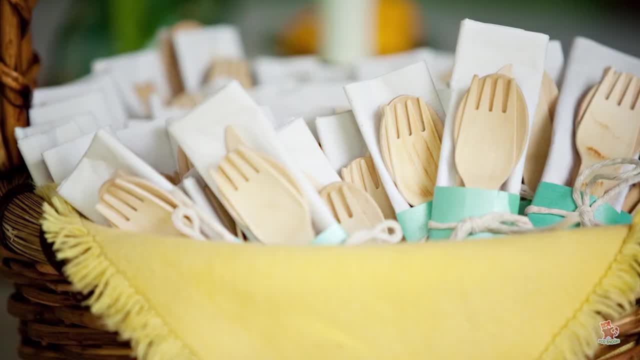 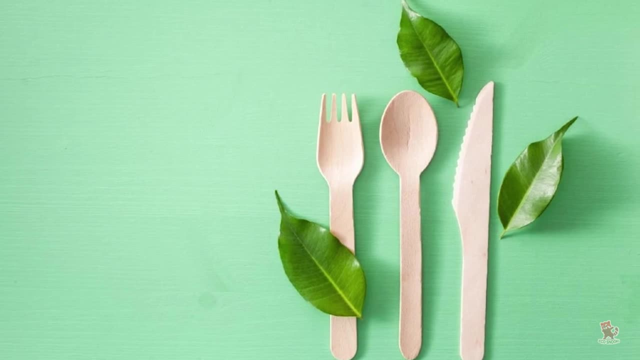 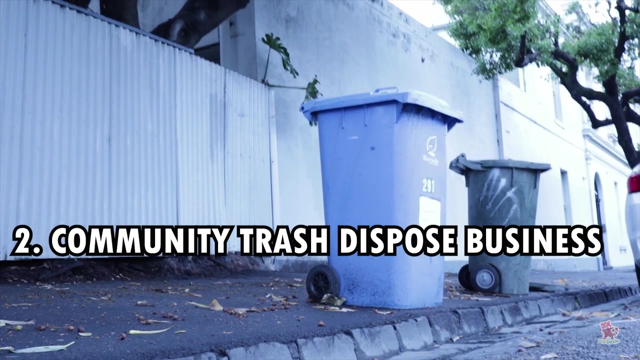 the plastic waste takes years to decompose. biodegradable cutlery is an environmentally safe alternative, usually made from bamboo. these forks, spoons, knives, plates and bowls are sturdy, robust, while being safe for the environment. trash needs to go somewhere, and large items like furniture and appliances can be particularly.